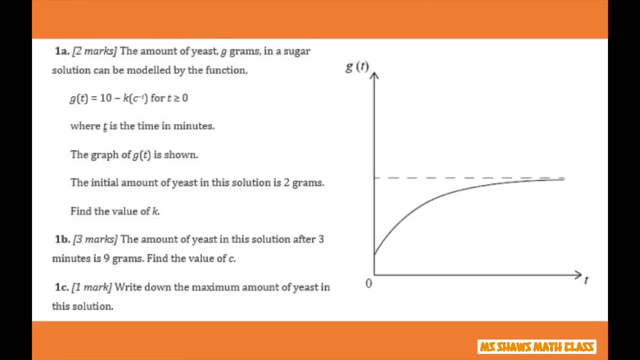 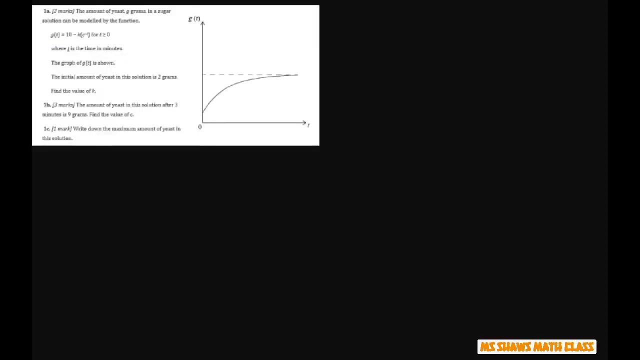 Hi everyone. The amount of yeast g grams in a sugar solution can be modeled by the given function. where t is the time in minutes, The graph is shown and the initial amount of yeast in this solution is 2 grams. Find the value of k. So let's do that first. 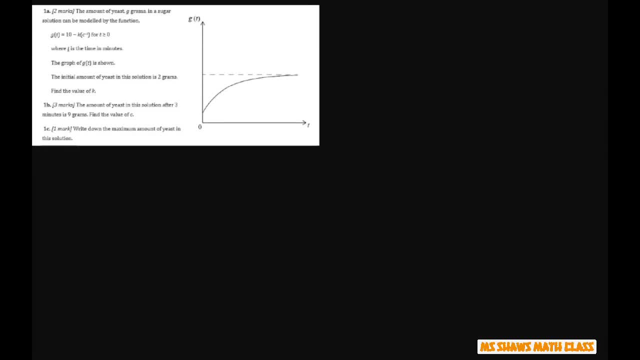 So all you're going to do is say the initial amount of solution is 2.. So that means 2 equals 10 minus k times c to the negative initial 0. So there's no negative, So you can just put c to the 0.. 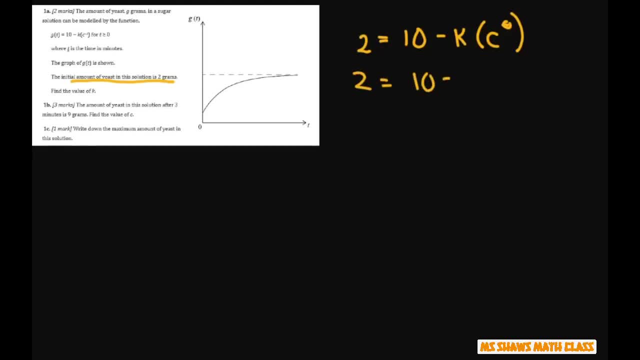 So basically you get 2 equals 10.. So 1 minus c to the 0, anything to the 0, power equals 1.. So 1 times k is just k Subtract 10. from both sides you get negative 8 equals negative k, So k equals 8.. 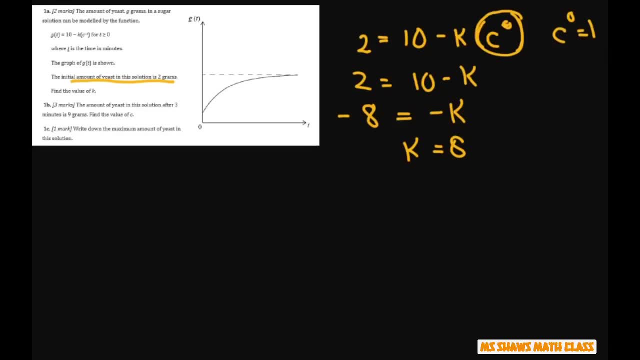 All right. So for b, it says the amount of yeast in the solution after 3 minutes is 9 grams. Find the value of g. So basically we're going to write our equation as: 9 equals 10 minus k. We already found k, which is 8 times c to the negative 3 power. 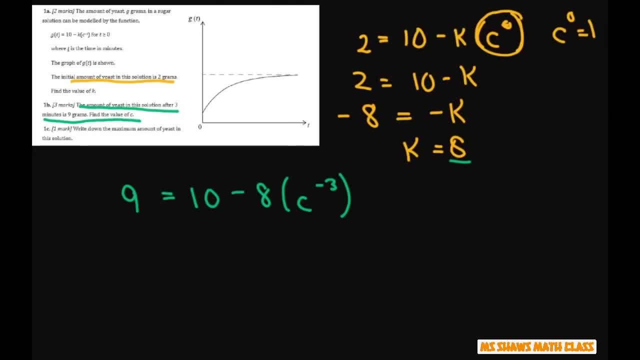 So simplifying that let's subtract 10 from both sides So you get negative 1 equals negative 8. So that's equal to negative 3 times c to the negative 3. I just subtracted 10 from both sides. 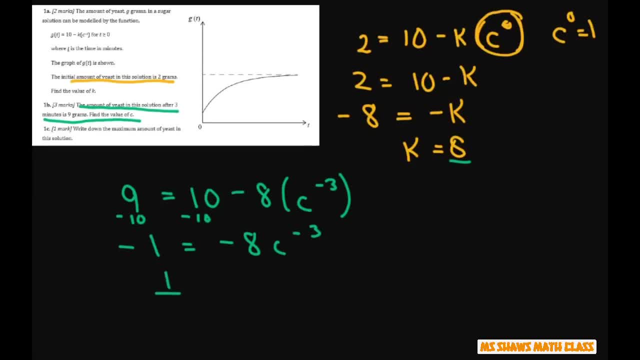 If you divide both sides by negative 8, you get 1 eighth equals c to the negative 3.. Now you can write this as 1 eighth equals 1 over c, cubed like that, Or you can write any of that.